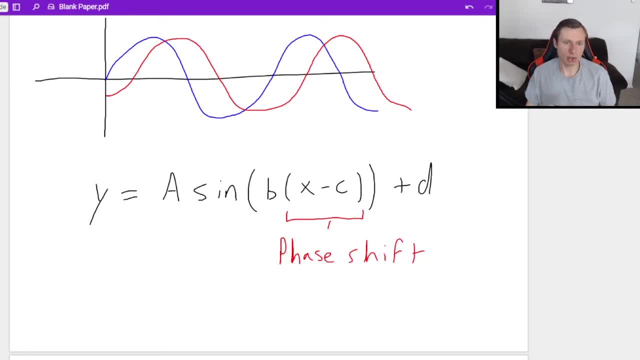 It's the x minus c part And basically what I'm saying is: let's say I have this equation, just something really easy: Y equals the sine of x minus pi over four. What that means is there is a shift of pi over four. shift pi over four to the right. 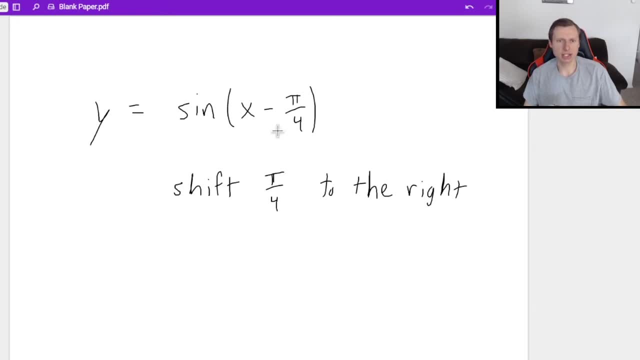 And why is it the right? Because this is clearly minus pi over four And that should be negative. left No For sine and cosine transformations. it's always the opposite of what you think. In other words, you see, minus pi over four, That means you shift to the right. 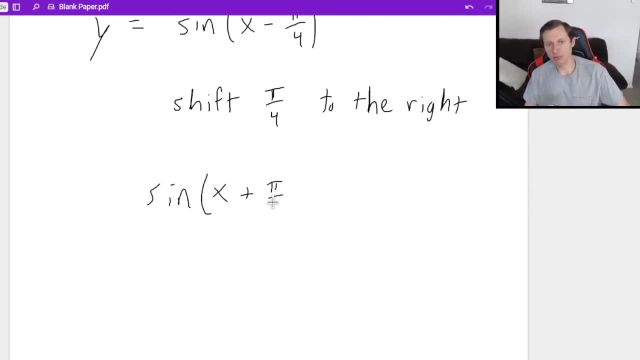 If you had the sine of x plus pi over four, that would be a shift to the left. It's always the opposite as what you think, And it's because, if we go back to the equation I drew earlier, it's not x plus c, it's x minus c, And that's what you think. And that's what you think, And that's what you think. 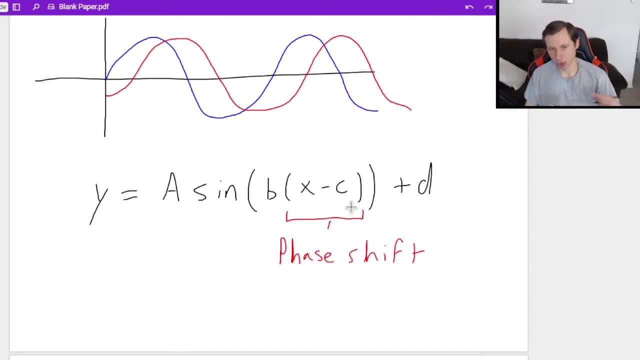 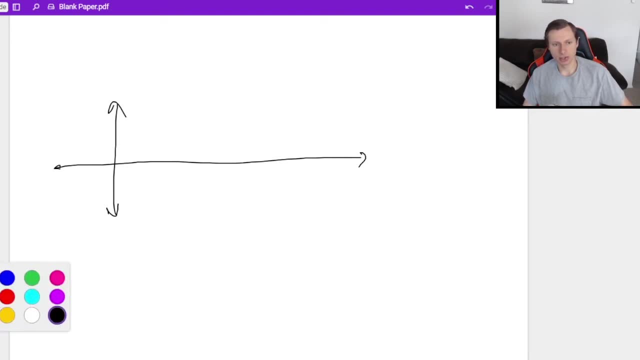 And that minus means that it's the opposite direction that you think it should be. Now what does the phase shift mean? What does a phase shift of pi over four even look like? I'll show you So again. here's my function. Looks something like this: Let's give you some. 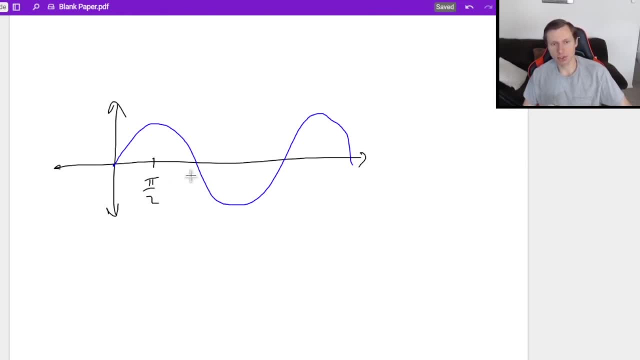 x values here like pi over two, pi three, pi over two and two pi. Now, if I'm shifting pi over four to the left- remember here is pi over four- But if I'm shifting to the left then I want negative pi over four. 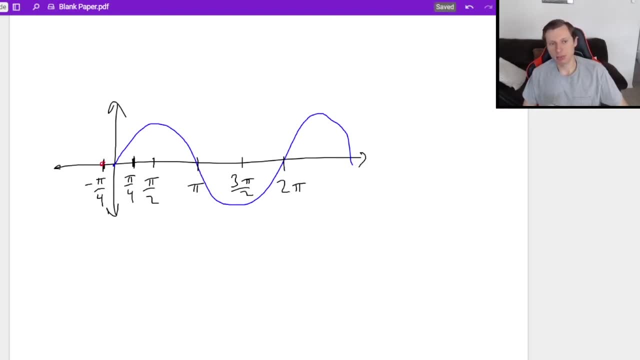 And here's what I'm going to do: I'm going to take my red, I'm going to put a dot at each of the points, a pi over four, right before it hits the blue. I have to be careful here And again. all of these red dots. 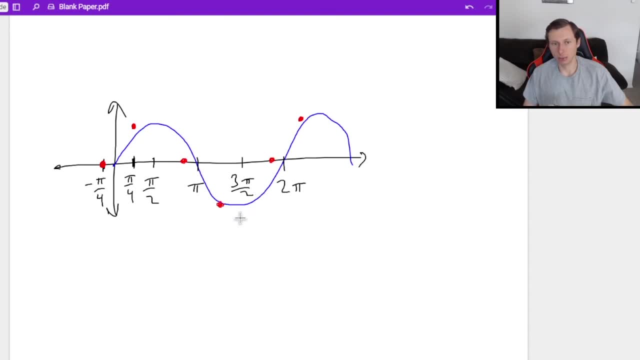 are pi over four to the left of the blue line. A lot of these I just guessed on. But as long as you're close, it's not going to matter. And if I just trace this out like I would a normal sine graph, there we go. That's what the graph is going to look like in red. 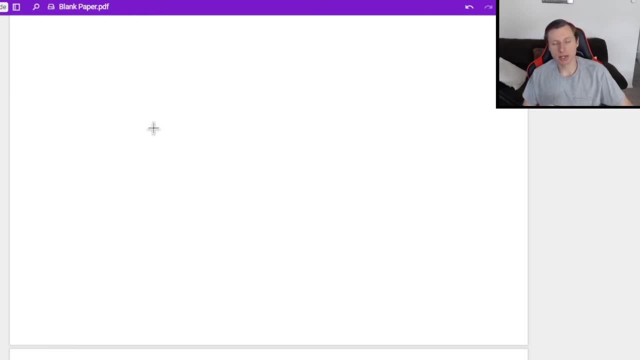 a shift of pi over four to the left. Now, by the way, there is something kind of weird with phase shifts, specifically with the period. Let me show you what I mean. If I have the graph, y equals the sine of x minus two pi. 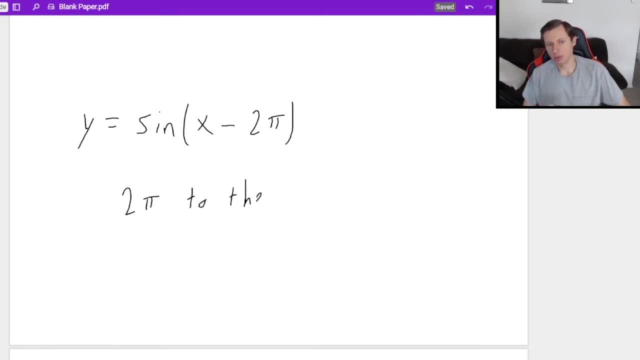 then again that's going to be a shift of two pi to the right. And if I remember how to find the period, well, the period of this sine function, what's in front of the x? it's nothing. So that means I follow the equation: period equals two pi over b. 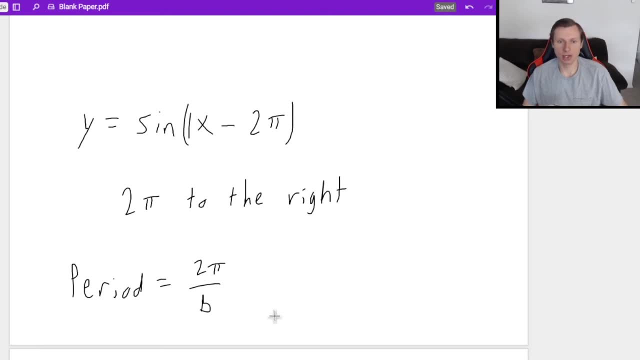 where b is the thing in front of the x. There's nothing there. It's technically a one. So the period is two pi over one. That means the period is two pi. So the period is two pi and I'm shifting two pi to the right. Something very cool happens when I do that. 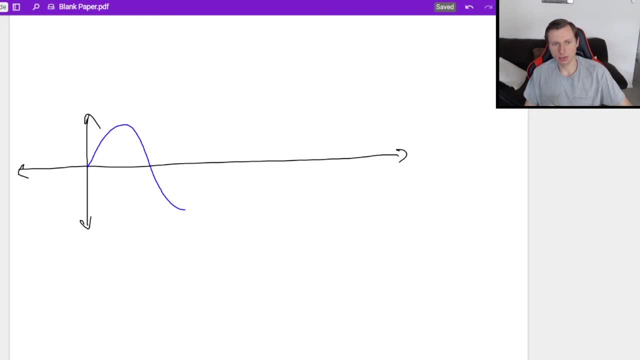 So first let me draw my sine graph in blue. Looks something like this. And remember, since the period is two pi, that means every time we hit here, here and here the same point on the sine graph, that distance is going to be two pi. 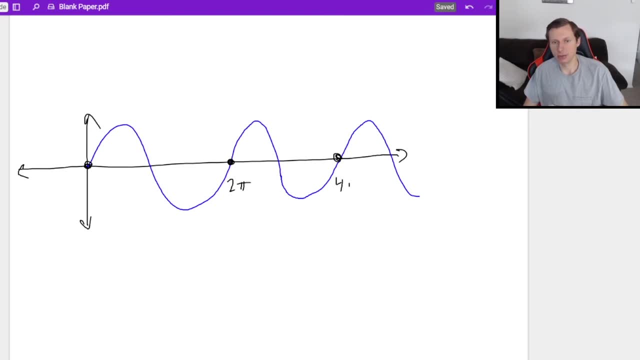 Like: right here is two pi, the second time it hits it four pi, and so on and so on. Now, if I'm shifting two pi to the right, I'm taking every point on the sine curve. So, for instance, this point right here, I'm taking it and shifting it two pi to the right. right there. 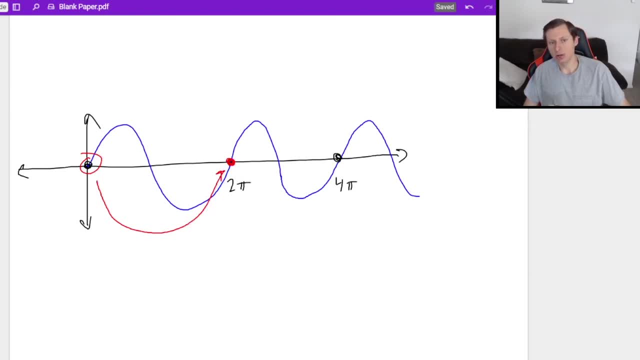 So this graph actually starts right here on that dot, and then it's just going to follow the sine graph And again, if I think of my points here, it's going to follow it exactly. My red is on top of the blue, and this is even true going the other way. 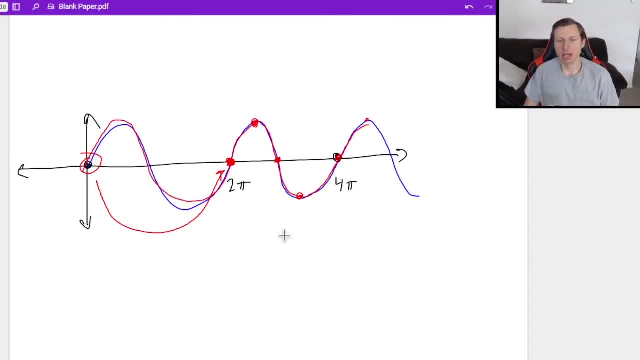 because sine technically goes both ways, left and right forever. It's going to line perfectly with my first graph. And why is that? Because the period was equal to the phase shift And whenever that happens, your graphs will look identical. You cannot tell them apart. 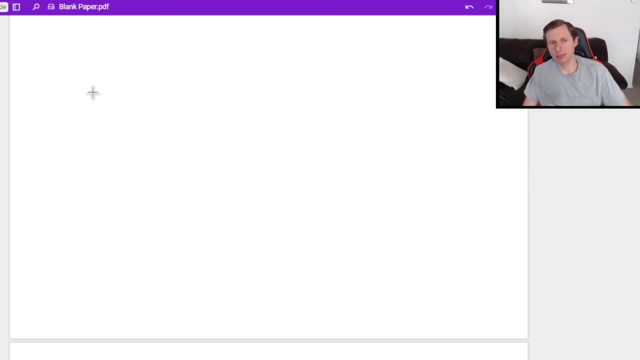 Now there's one more example I would like to look at today. It's the example where you see something like this: Sine of three x plus pi, something like this. Whenever you see this, the phase shift is not so easy anymore. 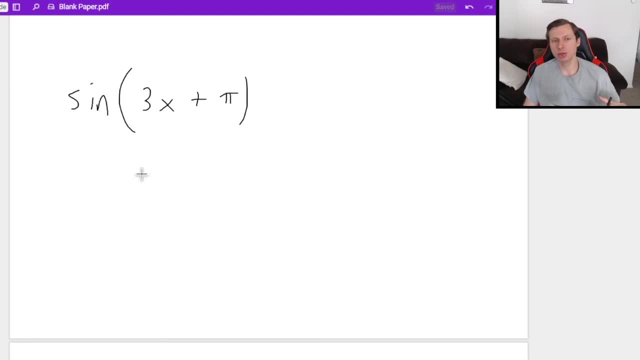 It's because of this three here. Basically, what you need to do is you need to factor out the three. Let me show you what I mean by that. So it's the sine of three x plus pi. So it's the sine of three x plus pi.